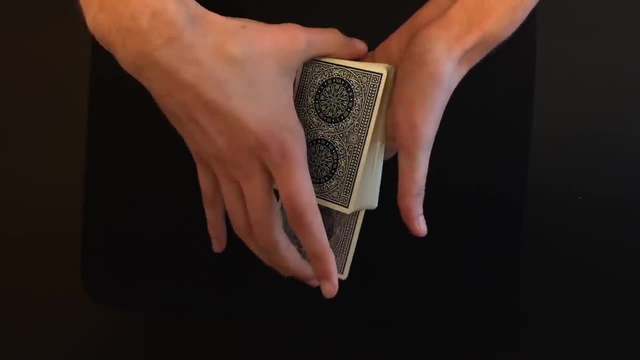 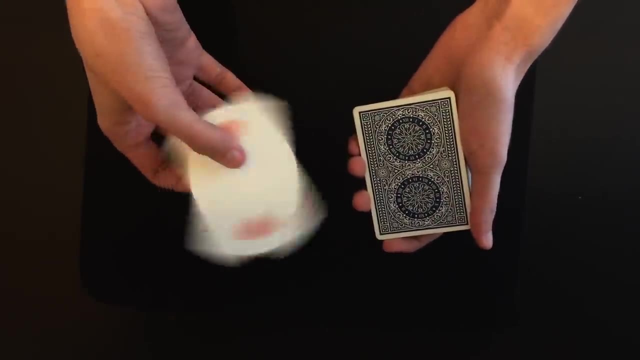 going to have the spectator insert their card anywhere they want, into the middle of the deck, just like this. So now their card is completely lost somewhere in the deck. Some people think that the card is like controlled at the top or something, but you guys can see it's really not. 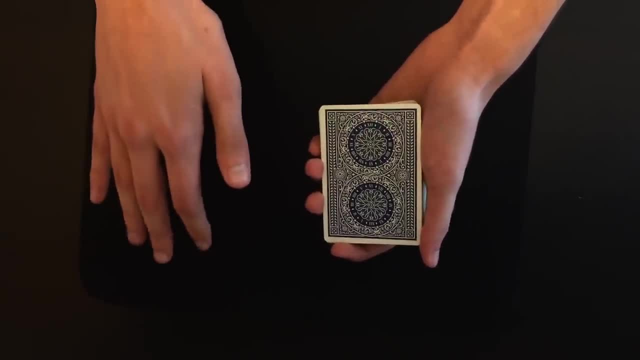 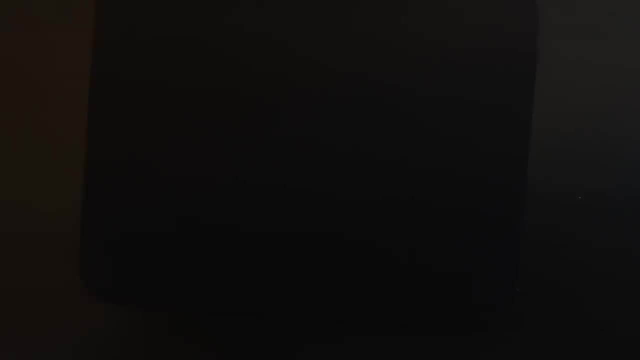 on the top. And now what I'm going to do is I'm going to go behind my back and I'm going to just make a little bit of a prediction, okay, And it'll be really quick, all right. So I think, yes, okay. 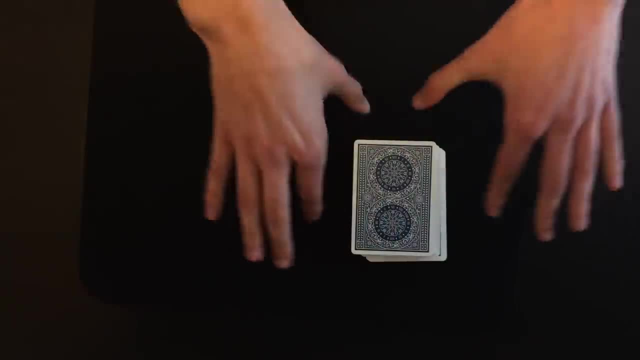 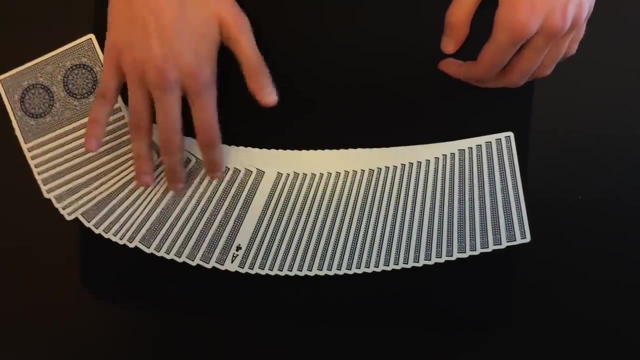 I think, okay, I got it. So what was the card that you picked? Interesting, because behind my back I took one card and I actually reversed it in the middle of the deck And you guys can see it is your card. 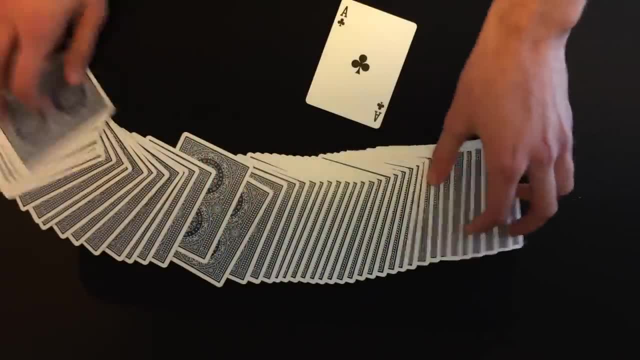 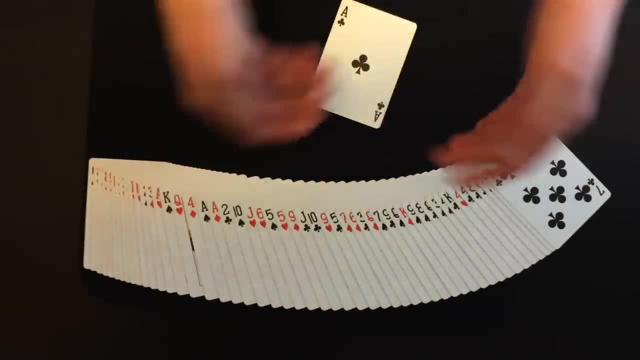 the ace of clubs And you guys can examine everything. All the cards here are normal and everything can be, you know, checked out by the spectator. So that is the trick, guys. and now for the tutorial. All right, guys, so here's the tutorial for the trick that you just. 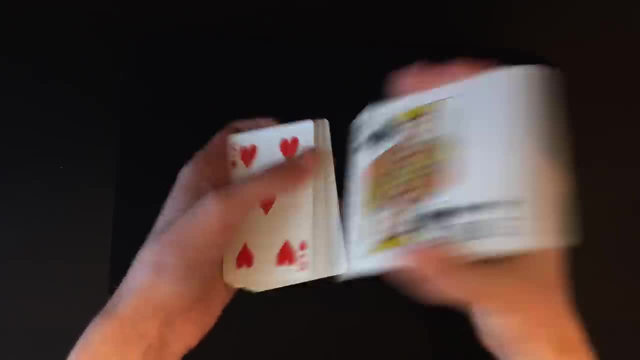 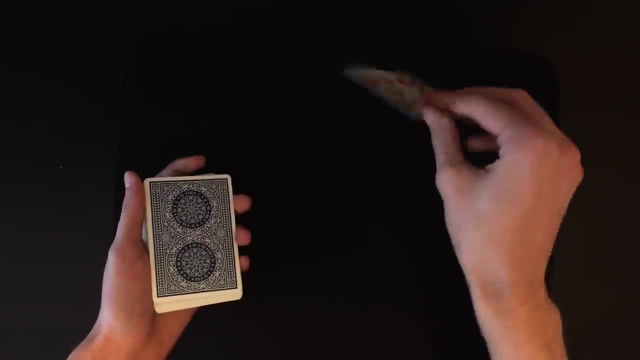 saw. So all you're going to need for this is just a normal deck of cards. It can be completely mixed up by the spectator. To start out the trick, you're going to have the spectator select any card. So they're going to pick out a card and they're going to look at it and they're 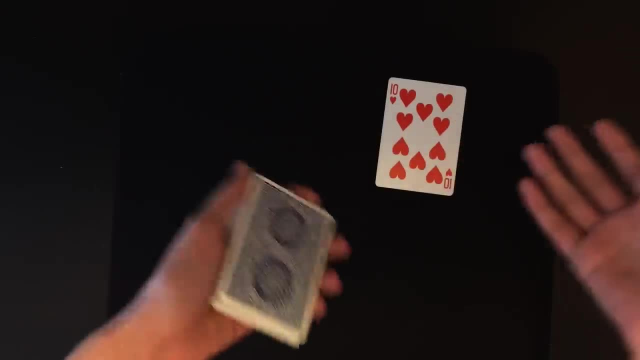 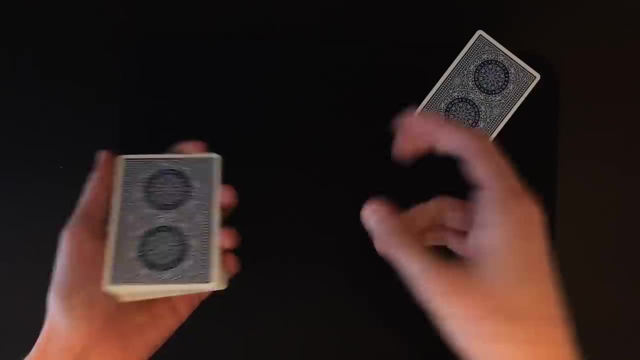 not going to be allowed to show you. So in this case, we'll be using the ten of hearts, and it's okay if I see it, because it's just the tutorial. So what's going to be happening is, while you give them the card, you're going to be turning around right, Because you know you don't want to see. 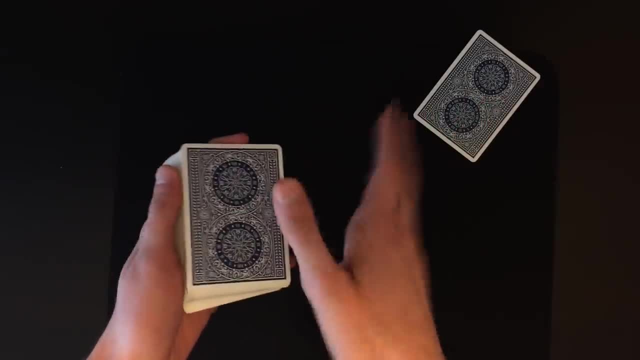 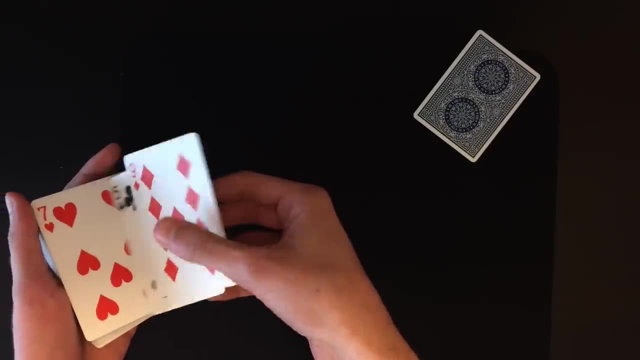 what the card is. But what you're actually going to be doing is just a little bit of a secret thing, and it's very, very simple. So what you're going to do, as your back is turned to the spectator, is you're going to just flip the deck over, take these two cards on the bottom. 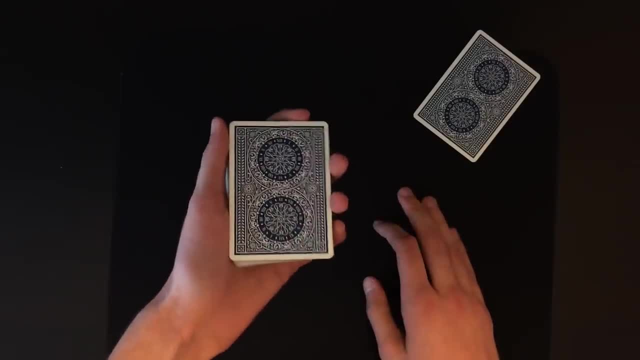 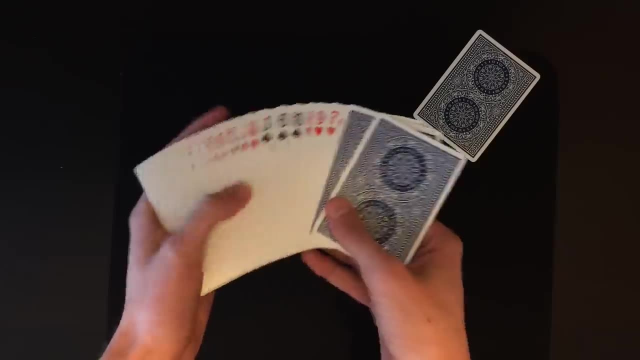 them over, and that's all you have to do. And now you can turn back around and come back to the spectator, and now you're in this position. So it looks like you just turned around and now you're back and the deck is exactly the same. What you've done is you've flipped over the two. 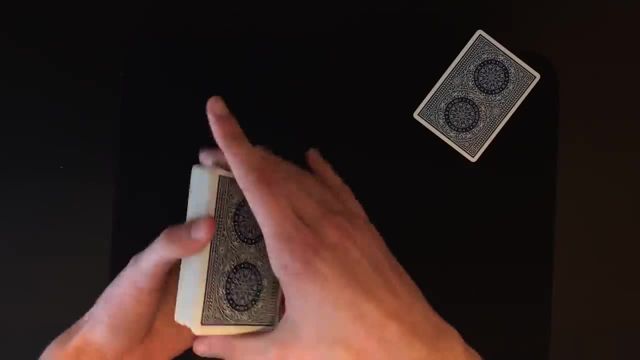 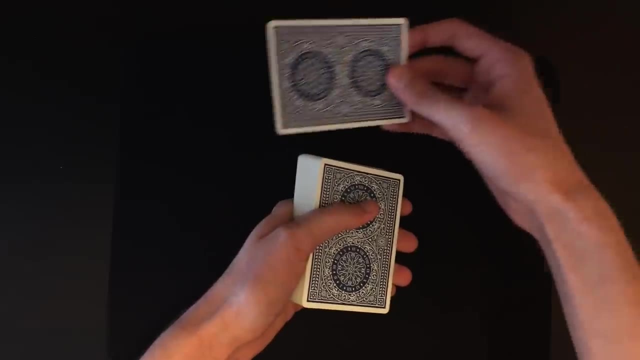 bottom cards and now the entire deck is face up. okay, So that's all you've done. But since the card on top is face down, the spectators think that the entire deck is face down. So now you're going to ask them to take the card and just kind of stick it anywhere they want to in the middle. 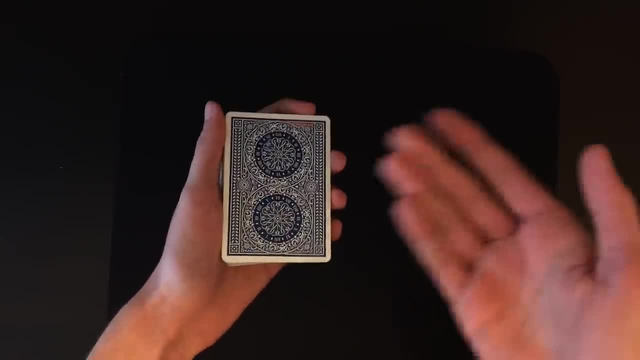 just like this, And they're going to do that, so they're going to push it in. and now you're going to say So. some people think that the card is like controlled to the top and all you're going to do is just spread off the top card. show it to them.